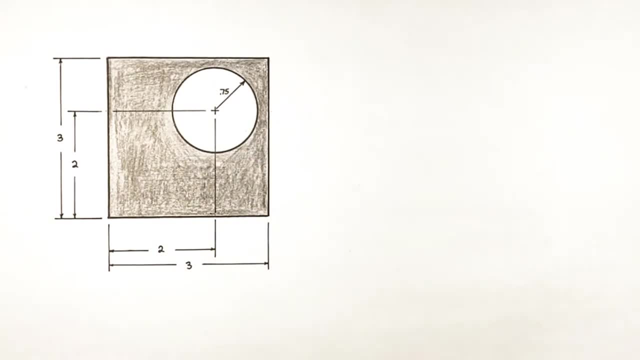 here the center of mass and the center of area in this case, are going to be the same. Now, anytime we're doing a center of mass problem, the first thing we need to do is establish some reference position or an origin, and the easiest place to do that is this bottom left corner right here. so 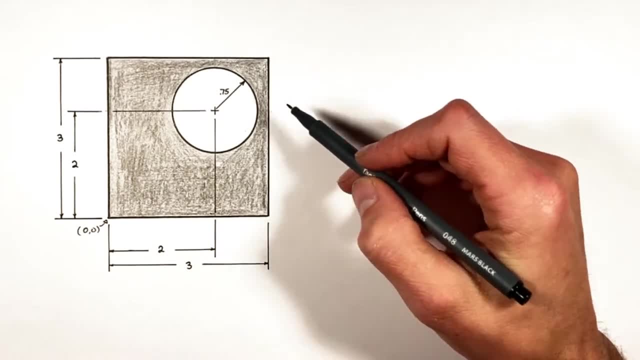 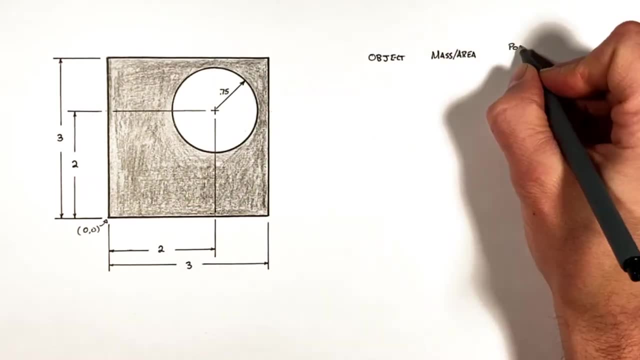 we're going to call this zero zero. Now to work out the center of mass, the first thing we're going to do is set up a table To keep all the information in this picture organized. so we're going to look at the object and the 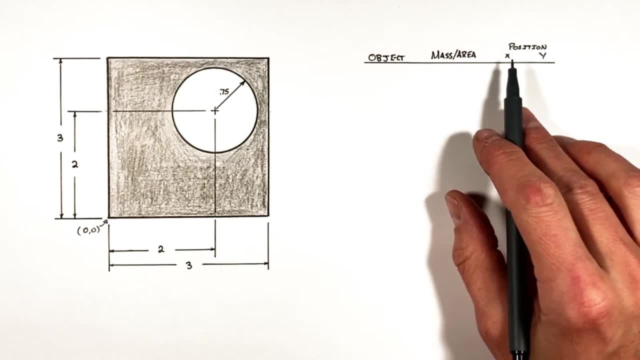 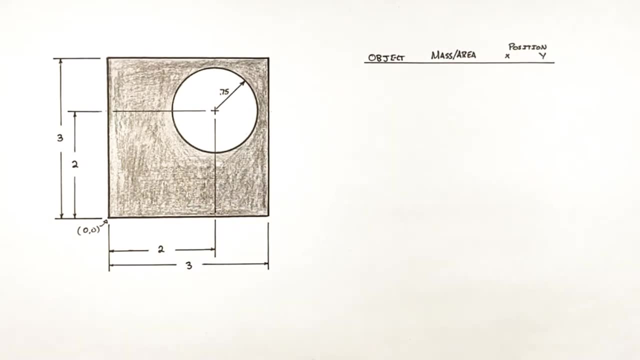 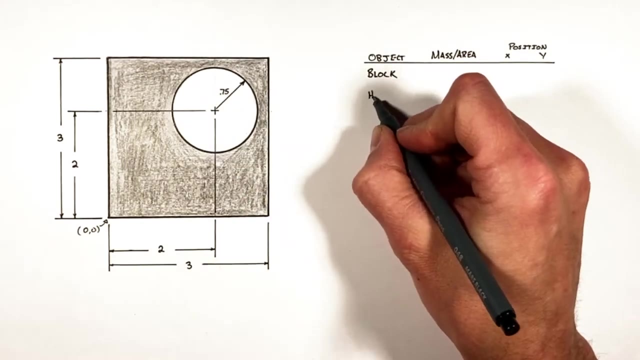 mass or area of each object, as well as each object's horizontal and vertical position. Now it looks like we only have one object, this block, but in reality there's actually two things here. The first is the block. The second object is the hole which we've cut out of the block and we don't know. 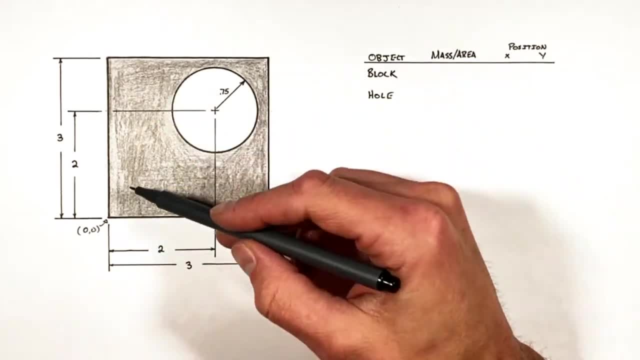 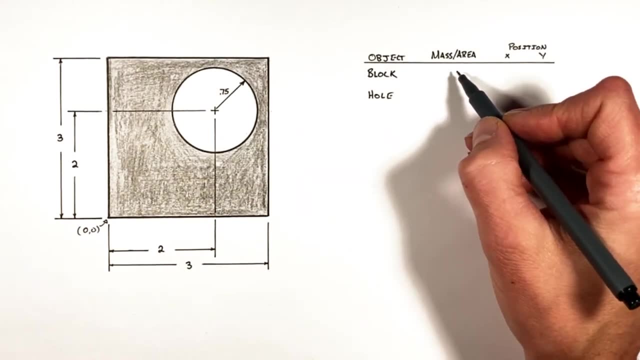 anything about the mass of this block. but what we do know is that if this material is of uniform thickness, then the mass and area are going to be proportional to each other. So, looking at this term here, for our area, the area of the block is simply going to be the base of the 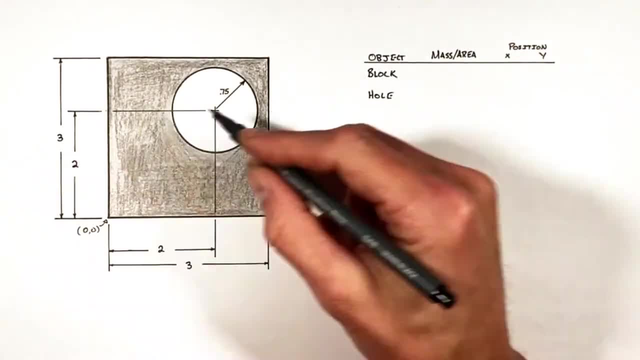 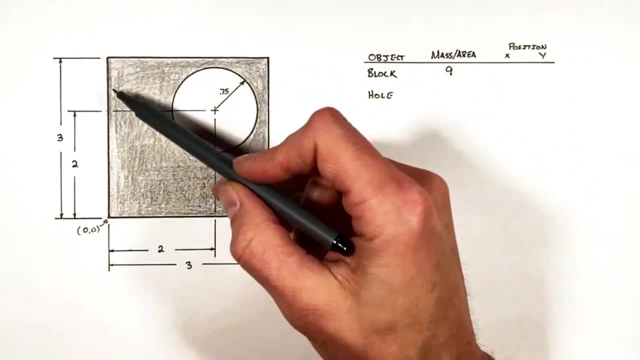 block multiplied by the height, That's three times three, which is nine. Now I know it's tempting to want to consider this hole here, but what we're first doing is looking at just the block as if there was no hole. We'll worry about the hole later. Now, looking at the center of area or center. 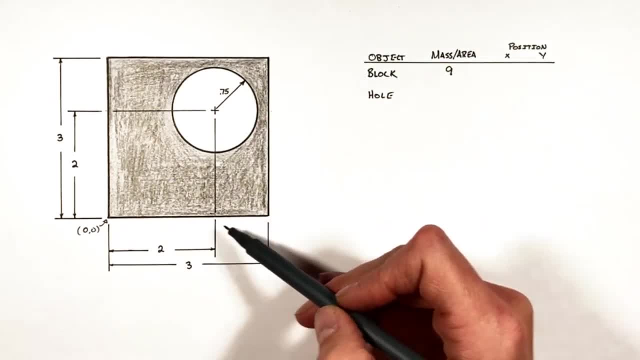 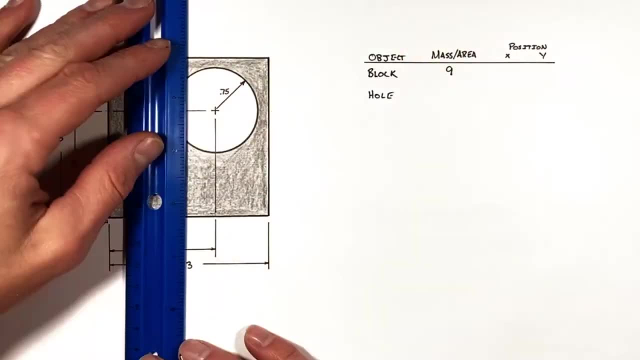 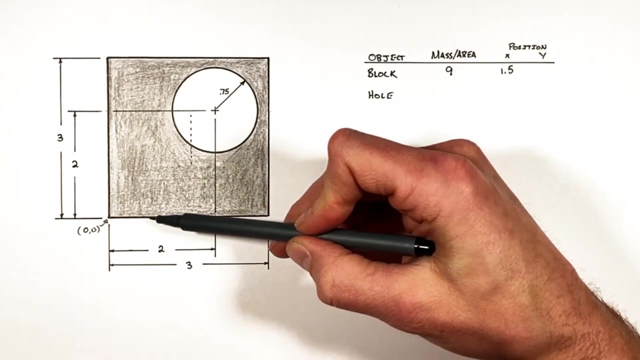 of mass of the block. We know, horizontally, the center of area or mass of the block is going to be halfway between the left and right edge of the block, So that's a position of 1.5. and vertically we see a similar thing. The center of mass or area vertically is half the height of the block, which is also 1.5.. 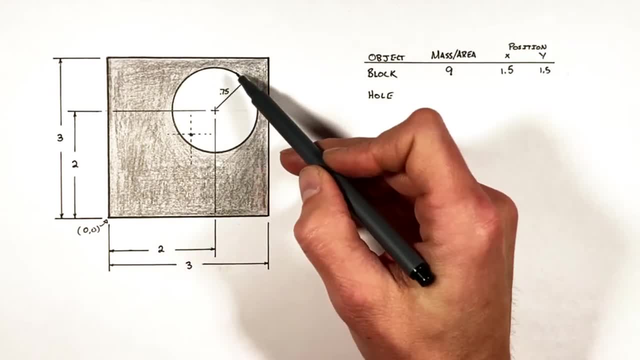 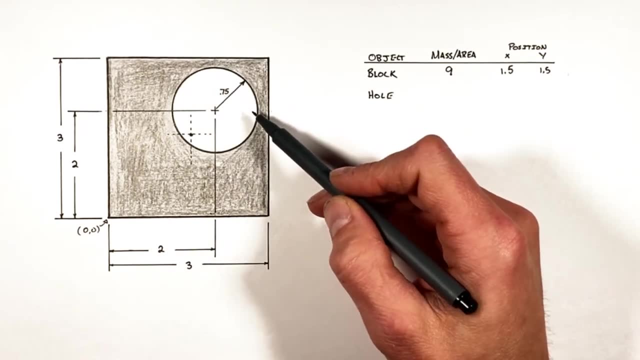 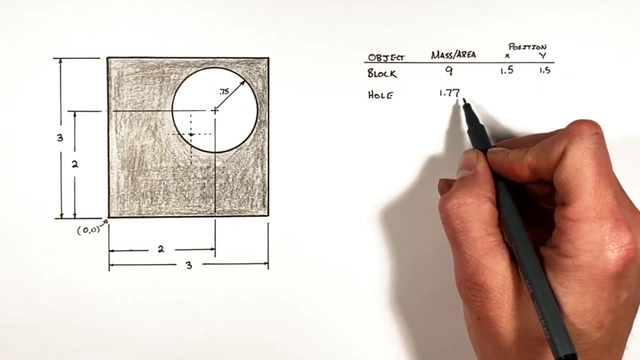 Now, working out our values for the block is pretty easy, but the hole is the, the key or the trick to the entire problem. See, when we remove this material, this hole has some area and, knowing the radius is 0.75, we can solve for that area And that area of the hole is 1.77.. But here's the trick, because we cut away. 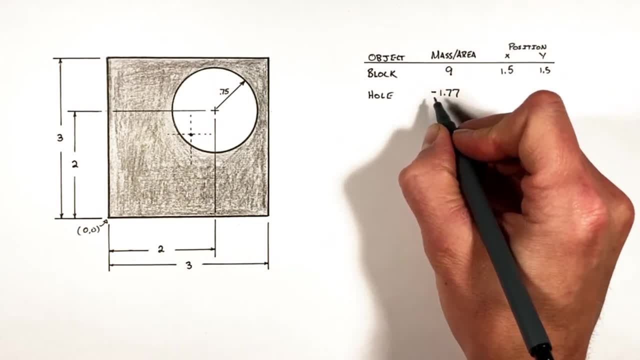 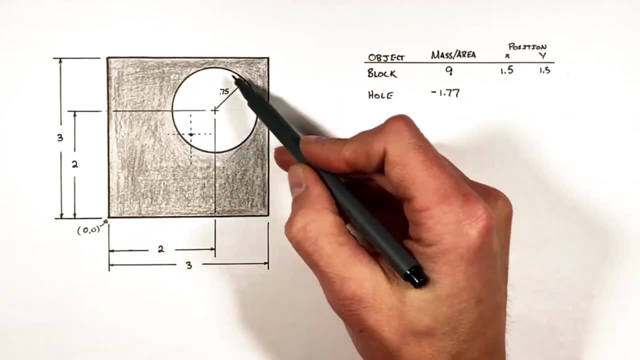 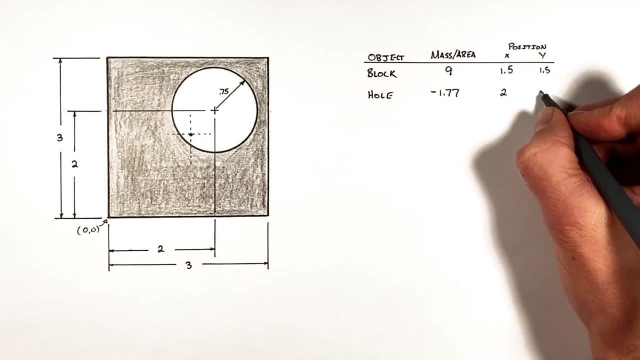 this material. this hole actually has a negative area. We've removed material. If we were to leave this positive, we would be saying we're actually adding extra material to this point. Now the hole is at a horizontal position. So we have a vertical position of 2 and a vertical position of 2.. Now our equation for center of mass. 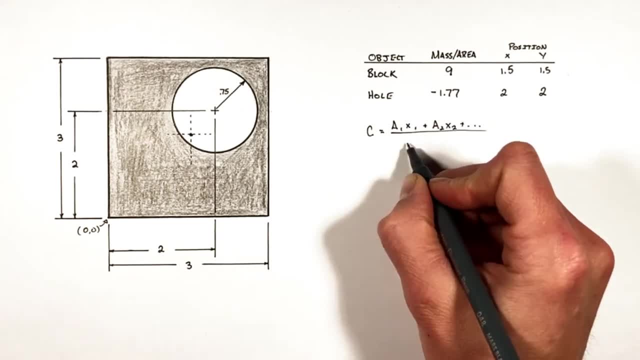 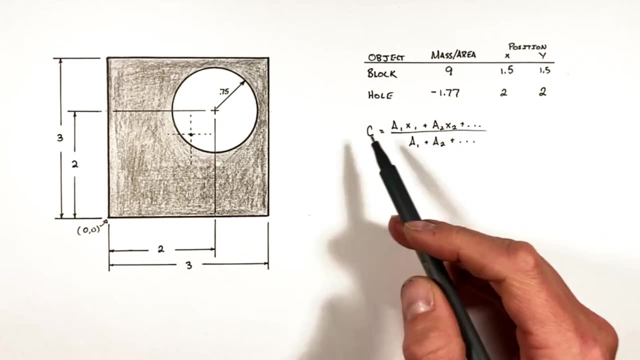 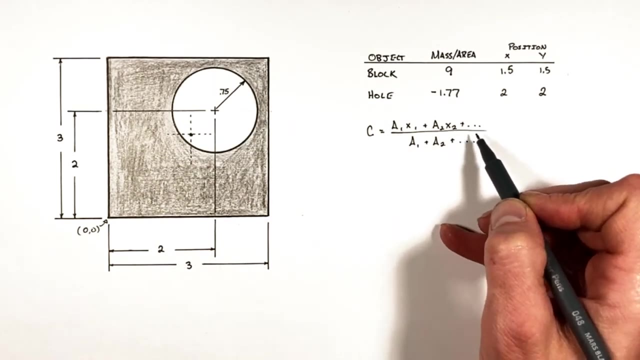 or center of area, is given by this equation. Now, technically speaking, if you wanted to solve for center of mass, you'd put in your values for mass here. But again, going back to the idea that the mass of this block is proportional to its area, we can interchange mass and area here without 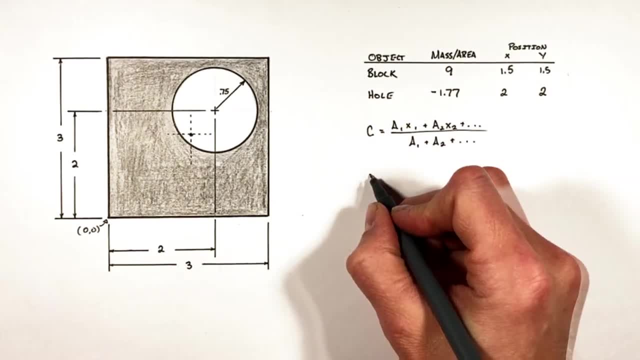 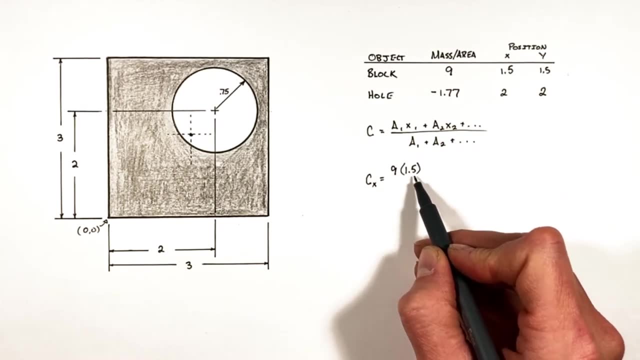 problems. So plugging in our values from our table into the equation. First, looking at the block itself, The block has an area of 9 and a horizontal position of 1.5.. The hole has an area of negative 1.77 and a horizontal position of 2.. 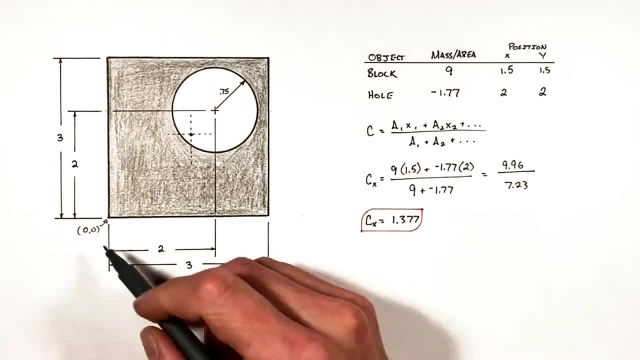 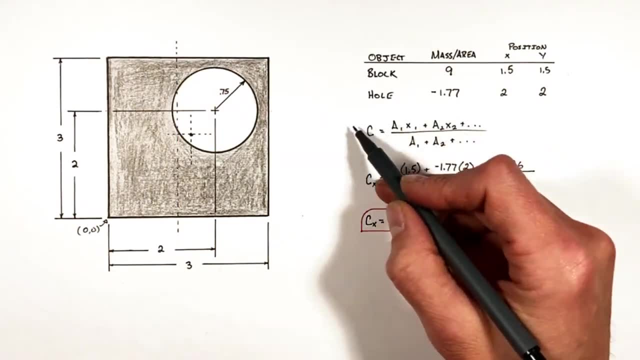 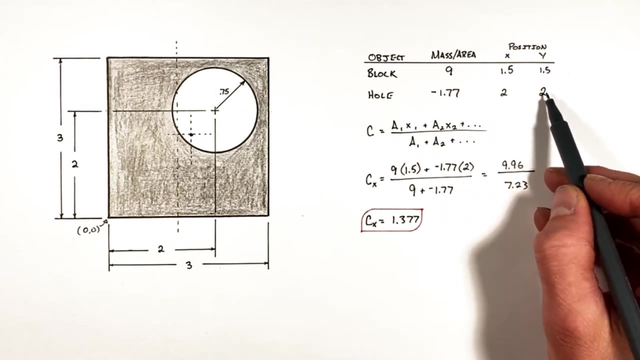 We find the center of mass in the horizontal axis is going to lie 1.377 to the right of our origin. Now we can do the same calculation using this equation for the vertical axis, Except, rather than plugging in our x values here, we can plug in the y values. But as you'll see, 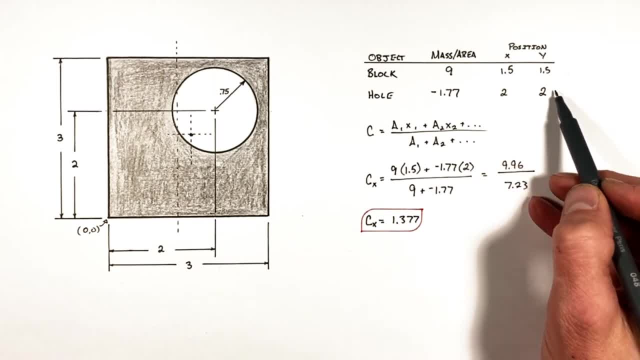 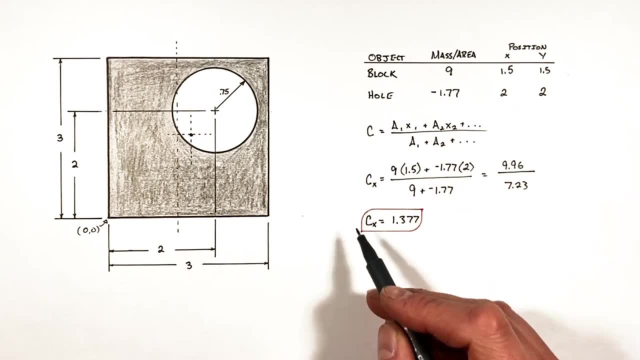 the horizontal and vertical positions for both of these objects are the same in both the x and y axis, Which means if we're to plug in these y values to this equation, we're going to get the same value for the center of mass or area in the y axis. 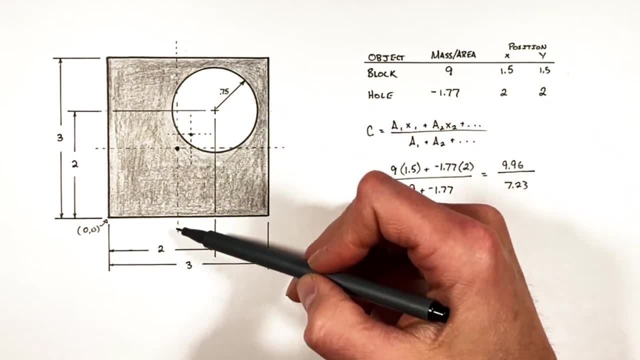 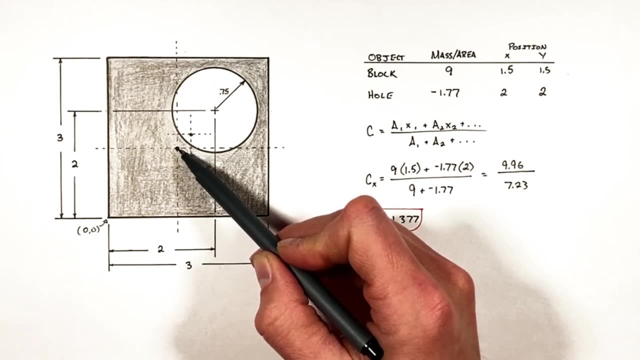 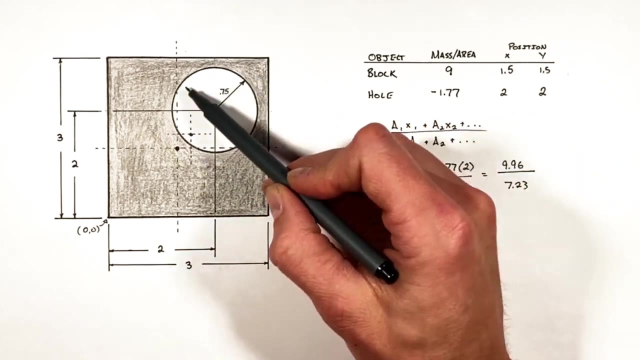 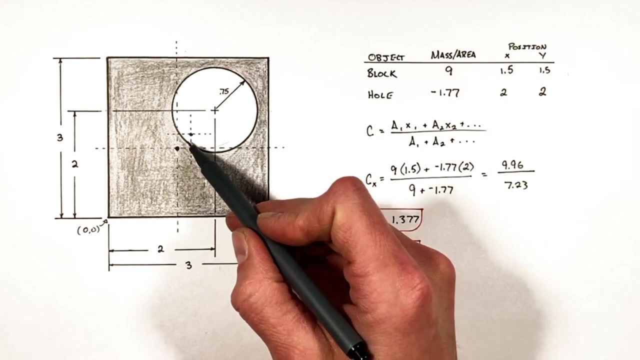 And that is given by that heat from the치� Fish in the hole needle. So looking inside here you can see, in this equation we want the center of mass of just the block to be BOB as well And we find in two dimensions the, the center of area of this block, with the hole fit. out of it lies right here. That's slightly below and to the left of where the center of mass of just the block was on its own. Think about it: if we were to remove material from the upper right corner of the block, that's gonna shift this center of mass or center of area down and towards the left, and that's exactly what we've seen here. Using a negative area, for this hole that was cut out of the rice is going to・ be огuirem Ngilds-made quark and washable under water. water for people watching. التي denver plants, up close to the line 4 and following the The Commander, A July 11 summer discussions began. 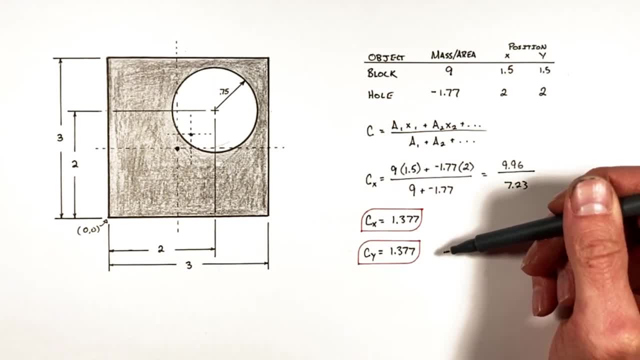 cut out of the block is what's called using a subtractive method of finding center of mass or center of area. I hope you found this useful and on that note, that's all for now.